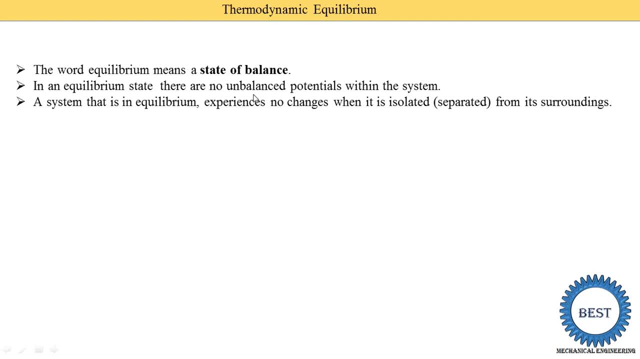 in equilibrium okay and it is isolated from the surrounding, is separate from the surrounding. at that time there is a no change in the system is occur okay. the system is said to exit in a state of equilibrium when no change in any macroscopic properties. okay means when there is a no change in a system in a macroscopic level means macro. 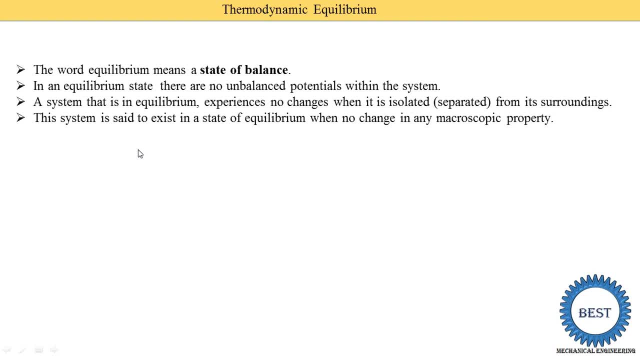 means on a very small level, there is a no change. then the system is said to be in a thermodynamic equilibrium. now here the exact definition of the thermodynamic equilibrium. a system is said to be in a state of thermodynamic equilibrium if the value of property is the same at all. the point in the system means we take the one any. 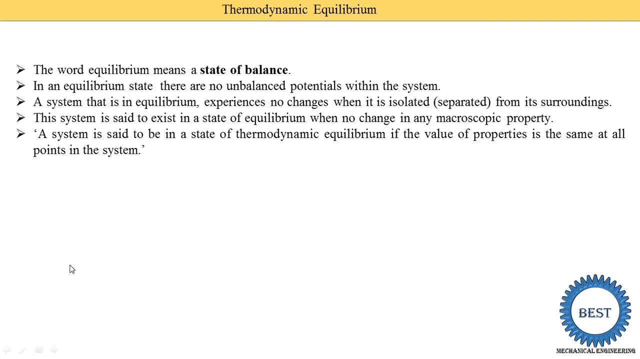 system and inside the system, at the every point, the property are same. it is called as the thermodynamic equilibrium. the system is said to be in a state of equilibrium if the condition for the following three types of equilibrium are satisfied: okay, so system is said in thermodynamic equilibrium if the three types of 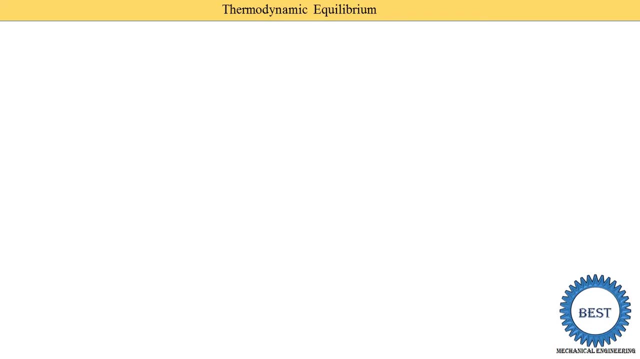 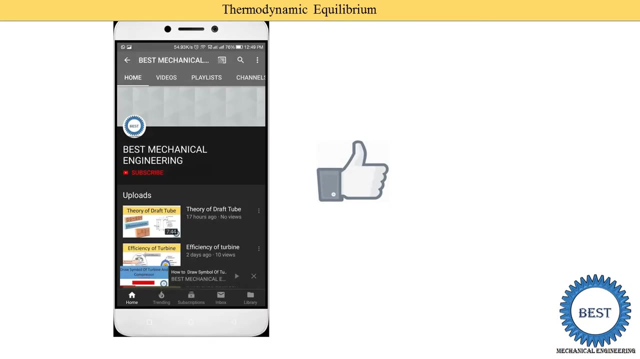 equilibriums are satisfied. now we focus on the what is the three types of the thermodynamic equilibrium. before that, i request to like the video and subscribe my channel for watching the more video related to thermodynamic subject, as well as for the another subject of the mechanical and. 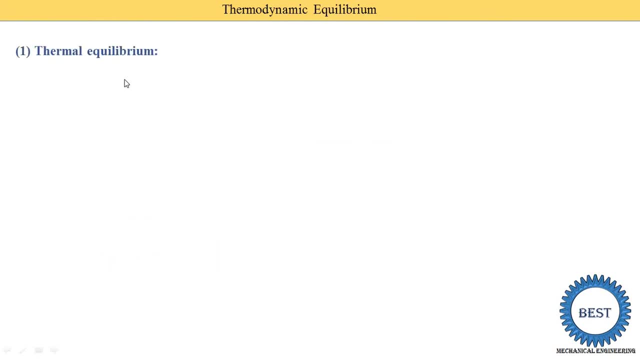 engineering. now, first we understand what is the thermal equilibriums. thermal means it is related to the heat, and heat is measured by using the temperature. okay, so if the temperature inside the system is equal, then it is called as the thermodynamic equilibrium. if the temperature of 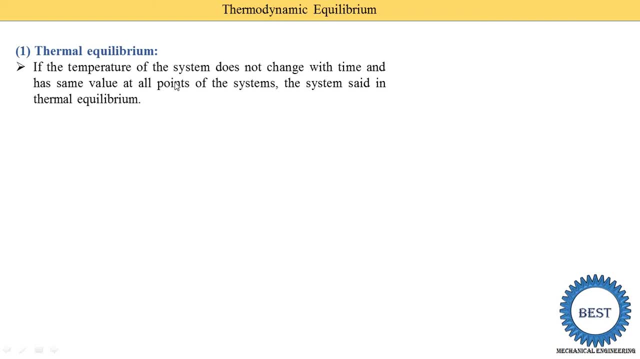 the system does not change with time means temperature not change with the time means temperature are same and same value at all. the point of the system. the system is said to be in a thermodynamic equilibrium. now, here you see, this is the two box. okay, so we consider this is our. 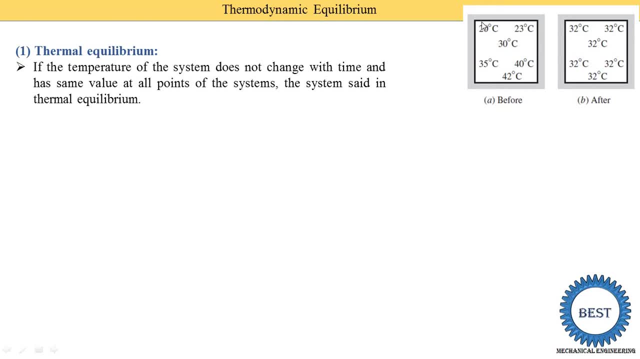 system. so in a first system that is a 20 degree temperature here 23, 30, 35, 40 and 42. so this system are not saying in thermodynamic equilibrium, because in the system at the different point there have a different temperature. so this first figure it is not in thermodynamic equilibrium. okay. 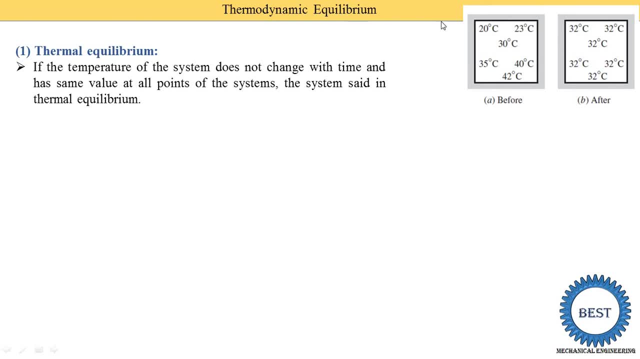 so this is the thermodynamic equilibrium and this is the thermodynamic equilibrium after, sometimes the this system is reached on to the thermal equilibrium, means after the thermodynamic equilibrium. here you see, temperature at the every point inside the system is the 32 degree centigrade, means these systems are in a thermal equilibrium. okay, similarly, second that: 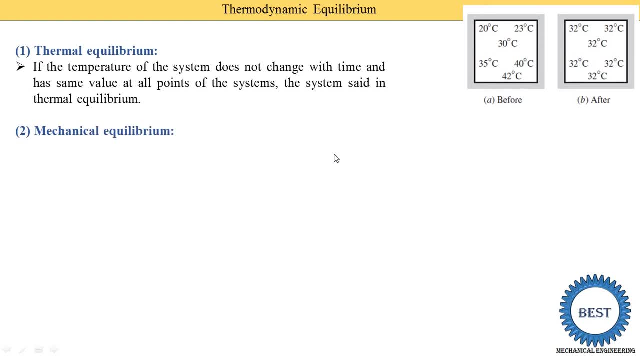 is a mechanical equilibrium. mechanical equilibrium is related with the pressure. okay, in this case, what we understand, temperature is different. okay, so if the system are not in thermal mechanical equilibrium, then the pressure inside the system is different at all the points. okay, the system are in mechanical equilibriums, then what the pressure inside the system is same. it is called as the 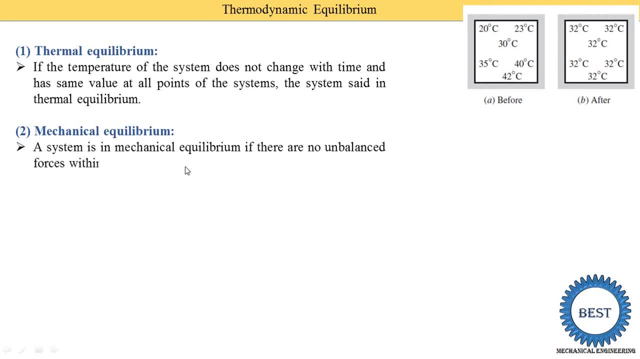 mechanical equilibrium. the system is in mechanical equilibrium if there are no unbalanced forces within the systems or between the surrounding. now forces means forces is directly depend on the pressure. pressure into area. force is equal to okay, so if the pressure is constant, then the force is also constant. okay, and the force is constant. that means the mechanical equilibrium is. 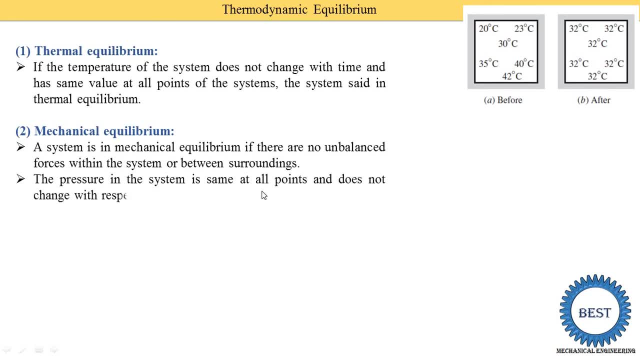 there, the pressure in the system is same at the all the point and does not change with respect to the time. now, here you see. this is the first system that is no mechanical equilibrium, okay, so here you see, if the pressure is different, that is 2 bar, 1 bar, 4 bar, 5 bar, 6 bar, okay, so, at every point there, 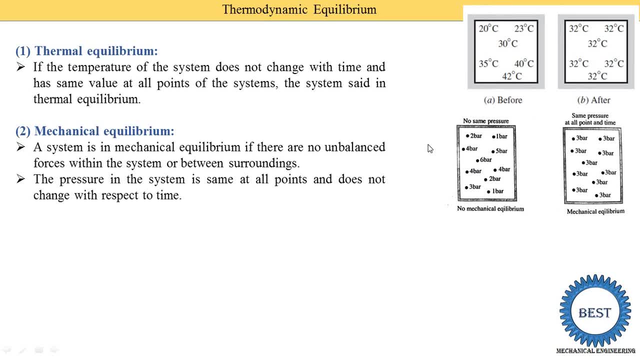 is a different pressure means there is a no same pressure, no same pressure. then the system is not in mechanical equilibrium. okay, now, here you see, the second system that are in mechanical equilibrium. why it is in mechanical equilibrium? because the pressure at the every point inside the system are 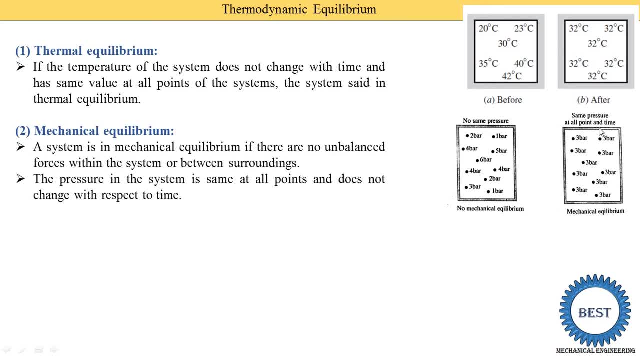 same, that is 3 bar, 3 bar, 3 bar. so same pressure at the all the point and the time. it is calling the mechanical equilibrium third system. is that sorry? third, thermodynamic equilibrium is chemical. it is chemical. composition does not change with the time. so according to name: chemical equilibrium. 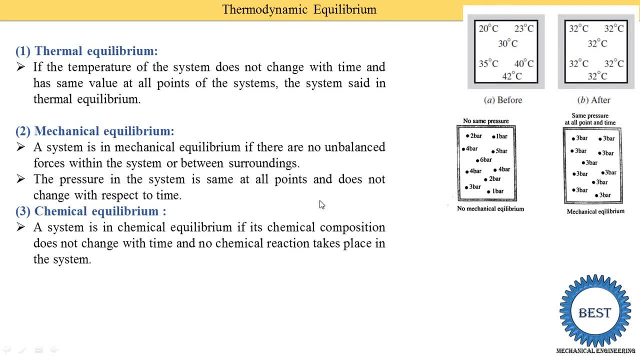 means they are required, the same chemical composition throughout the system and with respect to the time and no chemical reaction takes place in the system. it is called as the chemical equilibriums. now, here you see. this is a system one. so one point: that a carbon is present, some. 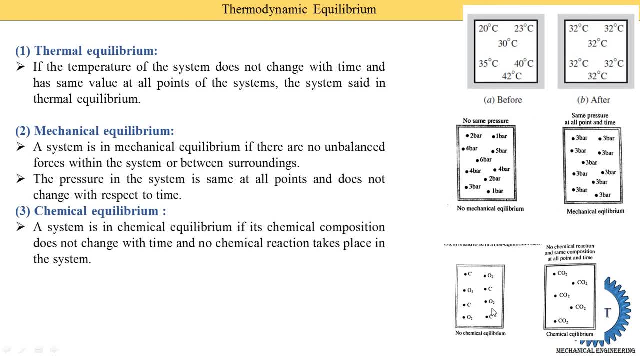 point though o2 is present. okay, so at the different point, that is, a different chemical is there and somewhere c is there, somewhere o is o2 is there, means carbon is there and the oxygen is there. okay, that is called as the no chemical equilibriums, but the some system is in chemical equilibrium, so a no. 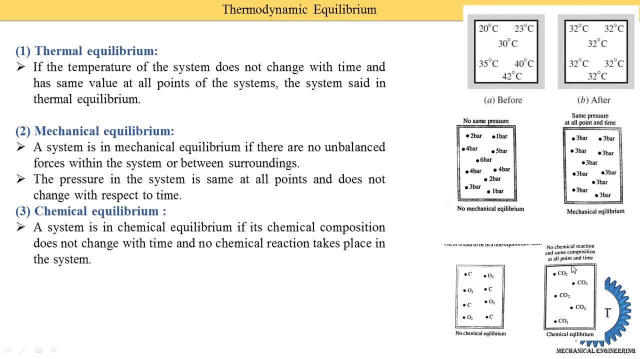 chemical reaction is there and the same composition at all the point in time. so here you see, this is a different point and at the all the point chemical composition is same. that is, the co2, that means the carbon dioxide, is there in the every point inside the system. that is called as the chemical equilibrium. 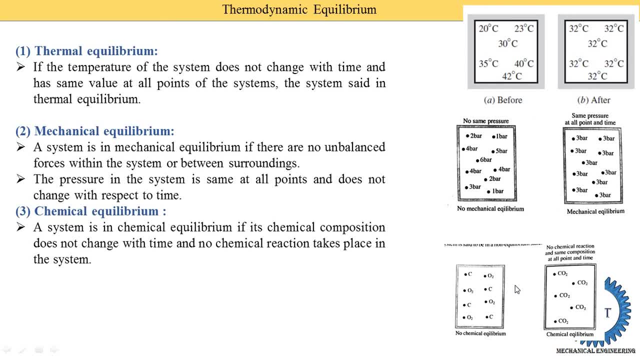 it is not that the chemical. sorry, chemical is the carbon dioxide. but there is a different refrigerant, is there? okay, suppose we talking about the vcrs system. so in a vcrs system there is a refrigerant is there that is r134, so its chemical composition is same. in a refrigeration, in compression means, 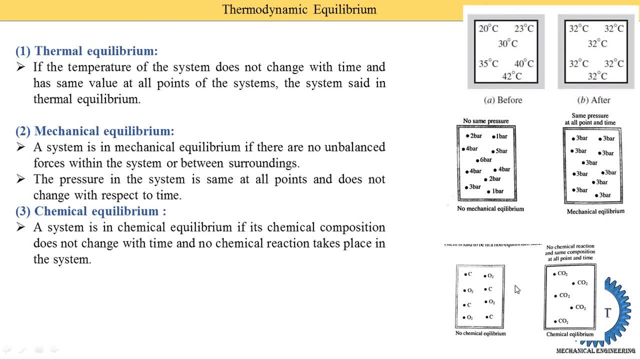 in condenser, in evaporator, and that okay. so this system is called as the in a chemical equilibriums. now, suppose the one system is satisfied, the lower equilibrium, thermal equilibrium, is there, because in a chemical equilibrium the system is not in carbonyl equilibrium or well, physically in equilibrium, but the system is not in chemical equilibrium. education momen achan bihed 놓al. 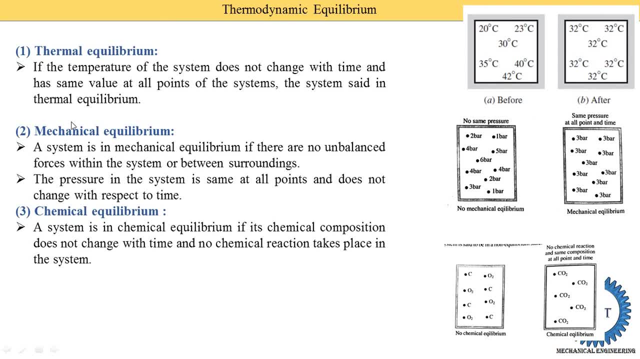 that okay. now system is in the chemical equilibrium and thermal equilibrium, but system is not in mechanical equilibrium. so system not followed. a thermodynamic equilibrium means system are not in the thermodynamic equilibriums. so here we written, when the above condition for any one of the three 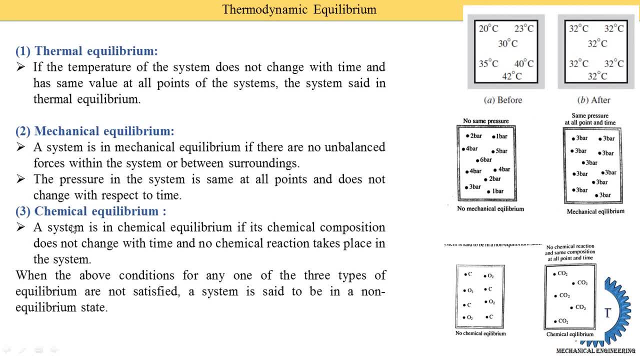 types of equilibrium are not satisfied means, out of three, any ones are not satisfied, a system is said to be a non equilibrium state. and if system is satisfy all these three equilibrium, then the system are said to be in a thermodynamic equilibriums. so thank you for watching this. 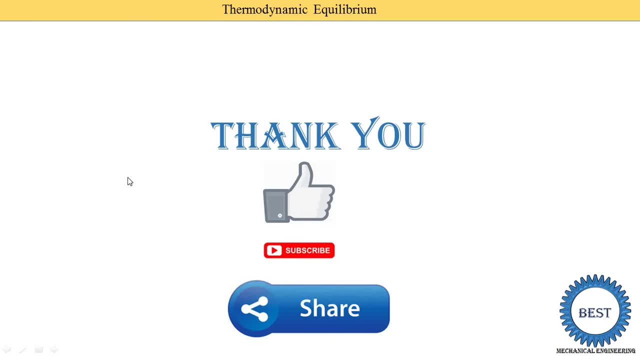 video. if you learned and like the video, subscribe the channels and don't forget to share with your friends.